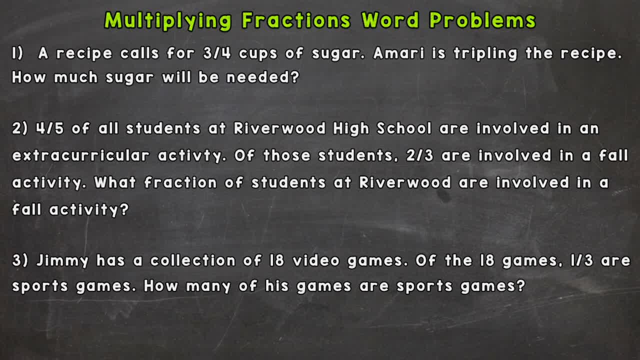 and how to solve. So let's jump right into number one, where we have a recipe calls for three-fourths cups of sugar. Amari is tripling the recipe. How much sugar will be needed? Well, Amari has three-fourths of a cup, right, And she is tripling. So that means to multiply by three. 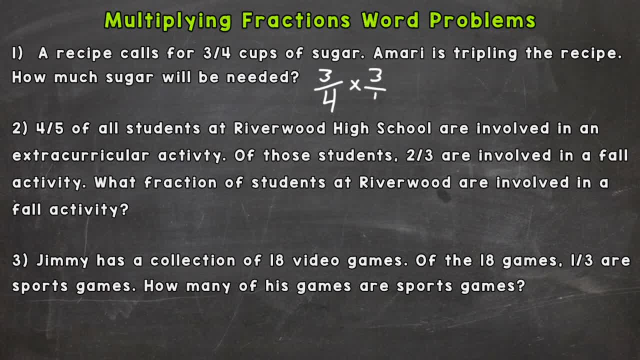 And I'm going to put my whole three over one. That way I have a numerator and a denominator. A whole number over one as a fraction is still worth that whole number. I'm not changing the value of the three Again, I'm just giving it a top and a bottom. That way I can multiply. 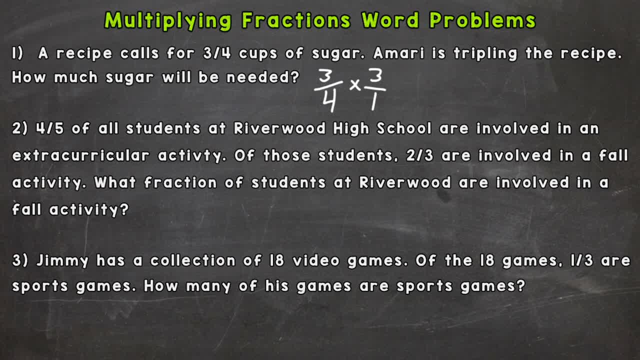 these fractions straight across. So three times three is nine and four times one is four. Now that's our answer, but it's improper, So we need to get it into a mixed number or maybe it works out To a whole number. So we need to do nine divided by four. How many whole groups of four can I pull? 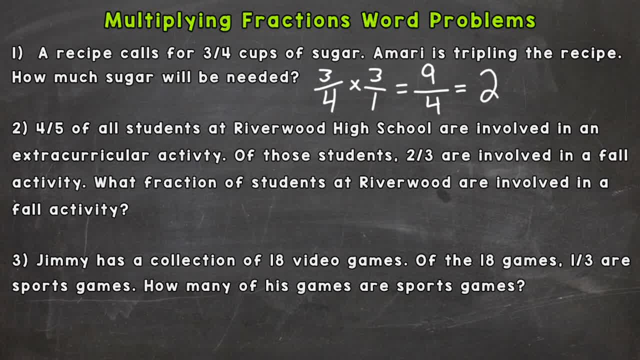 out of nine. Well, two, Two, whole fours. That gets me to eight. I didn't hit nine exactly, so I have a remainder of one and I keep my denominator of four the same. Since it's a word problem, I need to answer that question with a label here, and it's how much sugar will be needed. 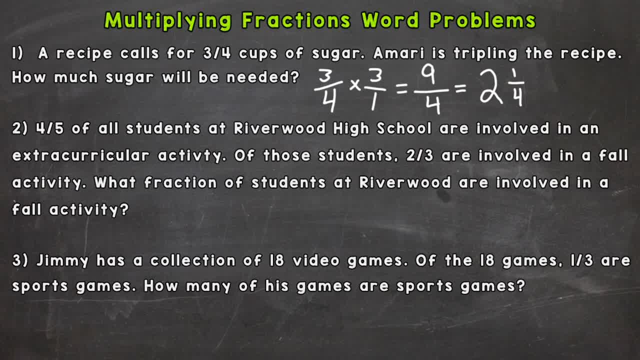 So we need two and one-fourth cups and that's our answer. So that example here would be a repeated addition type of multiplication problem. right, We needed three-fourths and we were tripling it. So three-fourths plus three-fourths plus three-fourths, which is just three-fourths times three. 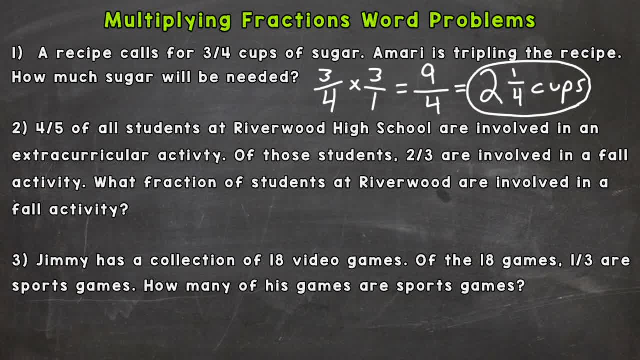 So let's take a look at number two, and we have a different type of word problem here. Four-fifths of all students at Riverwood High School are involved in an extracurricular activity. Of those students, two-thirds are involved in a fall. 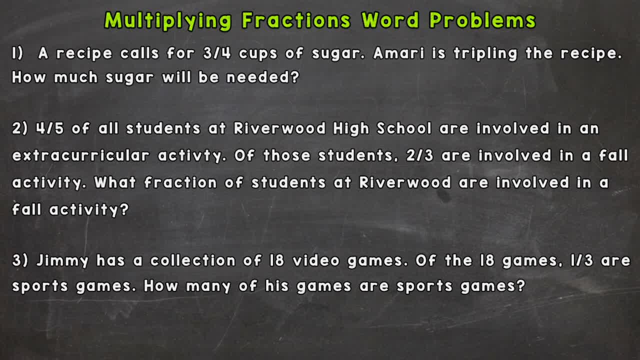 and how to solve. So let's jump right into number one, where we have a recipe calls for three-fourths cups of sugar. Amari is tripling the recipe. How much sugar will be needed? Well, Amari has three-fourths of a cup, right, And she is tripling. So that means to multiply by three. 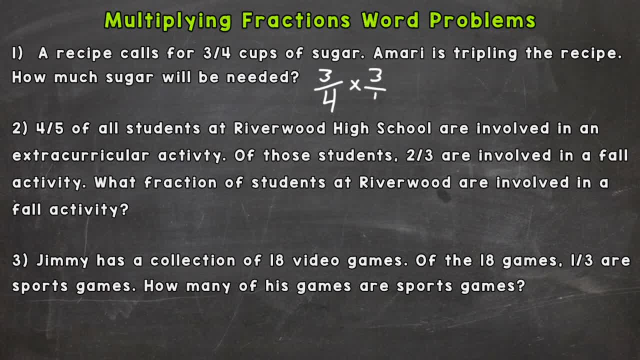 And I'm going to put my whole three over one. That way I have a numerator and a denominator. A whole number over one as a fraction is still worth that whole number. I'm not changing the value of the three Again, I'm just giving it a top and a bottom. That way I can multiply. 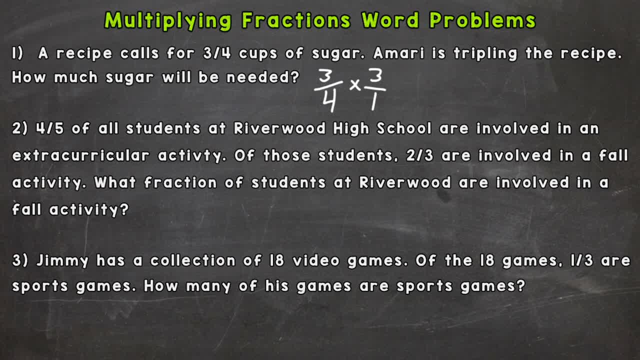 these fractions straight across. So three times three is nine and four times one is four. Now that's our answer, but it's improper, So we need to get it into a mixed number or maybe it works out To a whole number. So we need to do nine divided by four. How many whole groups of four can I pull? 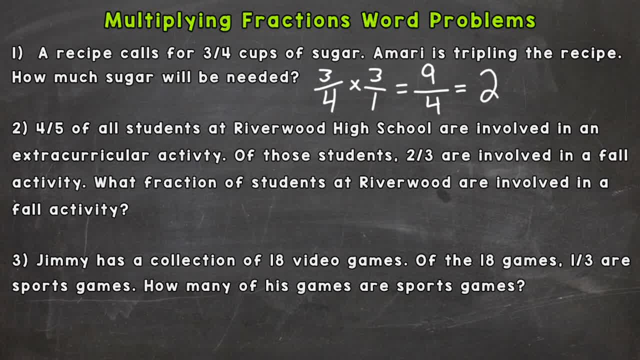 out of nine. Well, two, Two, whole fours. That gets me to eight. I didn't hit nine exactly, so I have a remainder of one and I keep my denominator of four the same. Since it's a word problem, I need to answer that question with a label here, and it's how much sugar will be needed. 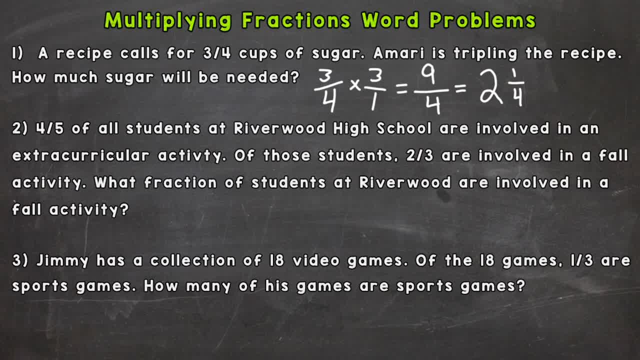 So we need two and one-fourth cups and that's our answer. So that example here would be a repeated addition type of multiplication problem. right, We needed three-fourths and we were tripling it. So three-fourths plus three-fourths plus three-fourths, which is just three-fourths times three. 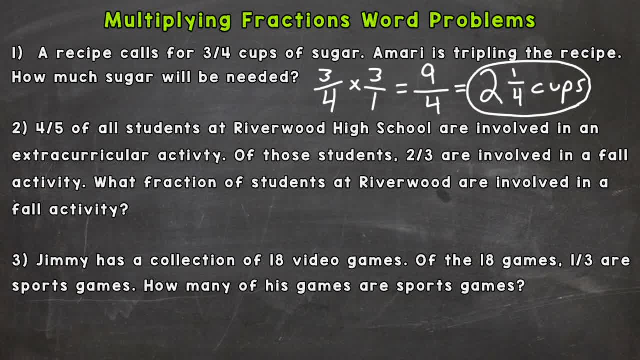 So let's take a look at number two, and we have a different type of word problem here. Four-fifths of all students at Riverwood High School are involved in an extracurricular activity. Of those students, two-thirds are involved in a fall. 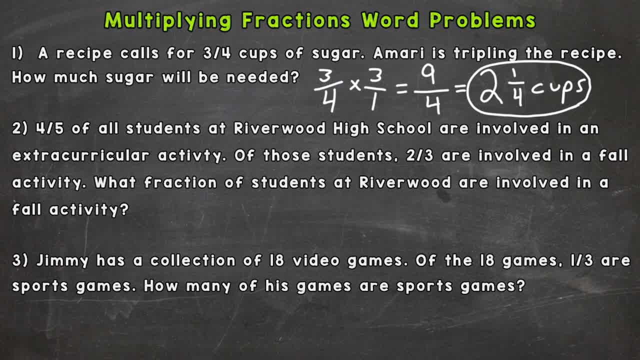 activity. What fraction of students at Riverwood are involved in a fall activity? So here we have a fraction of a fraction problem. So what fraction of students at Riverwood are involved in a fall activity? So what fraction of students at Riverwood are involved in a fall activity? So here we have a fraction of a fraction problem, where we're taking a fraction of a fraction. 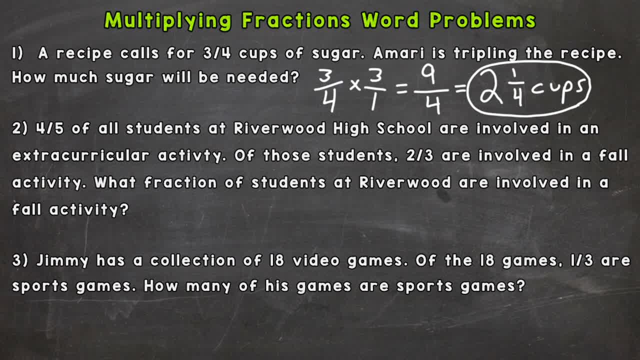 So whenever we have any of these of problems, whether it's a fraction of a fraction, fraction of a whole number or fraction of a mixed number- we can use multiplication to solve. So in this situation, we're taking two-thirds of four-fifths, and that will give us our answer. 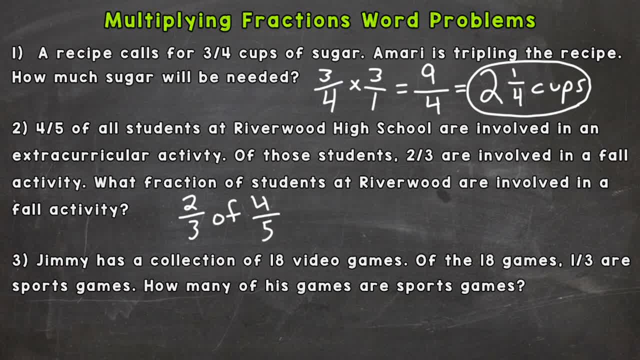 So in this situation, we're taking two-thirds of four-fifths and that will give us our answer, And we can just replace that of with a multiplication sign. We can use multiplication to solve here. So I'm going to rewrite the problem: Two-thirds times four-fifths. 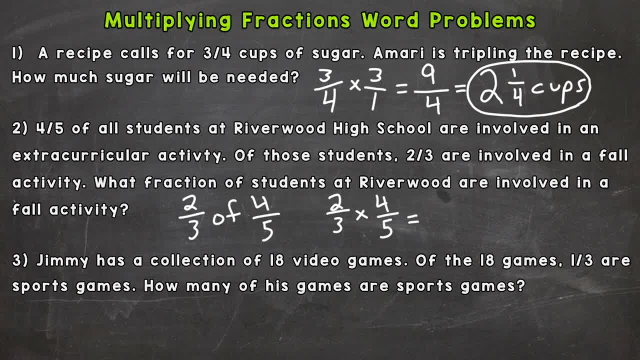 Now I can multiply straight across: Two times four is eight. Three times five is fifteen. That fraction's in simplest form. so now we need to put a label, And our question was what fraction of students at Riverwood are involved in a fall activity? 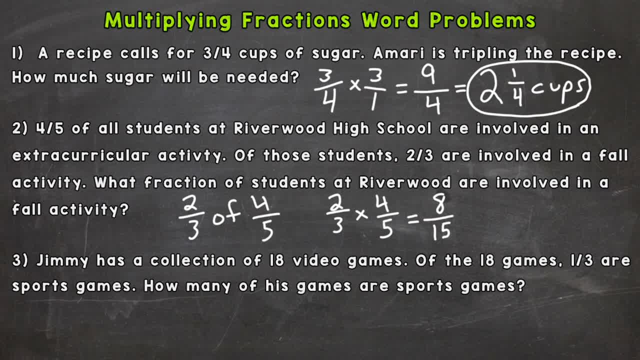 So eight-fifteenths of students are involved in a fall activity. So again, that was a fraction of a fraction type of problem. Now number three is going to be similar to number two, but it's going to involve a whole number and a fraction. 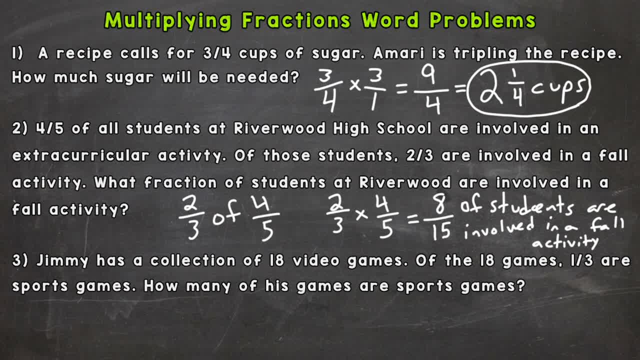 So Jimmy has a collection of eighteen video games. Of the eighteen games, one-third are sports games. How many of his games are sports games? Well, much like number two. we're taking a fraction of something We're taking. one-third of his eighteen video games are sports games. 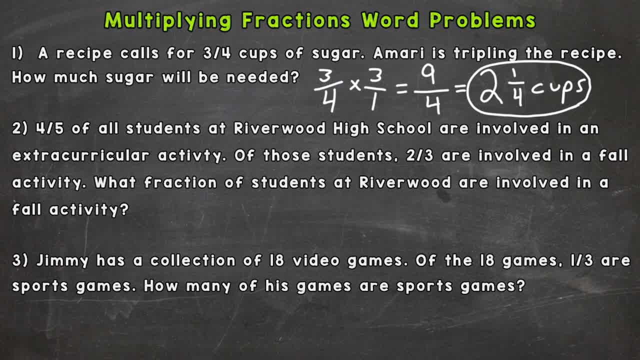 activity. What fraction of students at Riverwood are involved in a fall activity? So here we have a fraction of a fraction problem. So what fraction of students at Riverwood are involved in a fall activity? So what fraction of students at Riverwood are involved in a fall activity? So here we have a fraction of a fraction problem, where we're taking a fraction of a fraction. 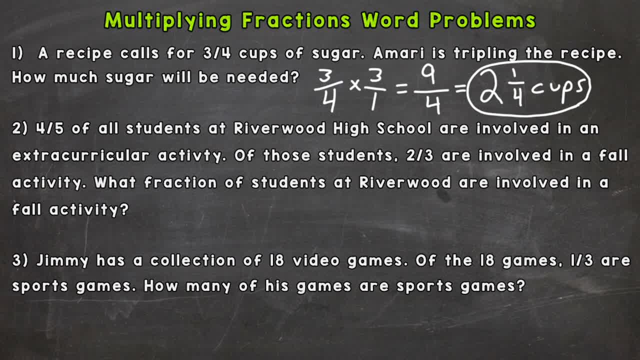 So whenever we have any of these of problems, whether it's a fraction of a fraction, fraction of a whole number or fraction of a mixed number- we can use multiplication to solve. So in this situation, we're taking two-thirds of four-fifths, and that will give us our answer. 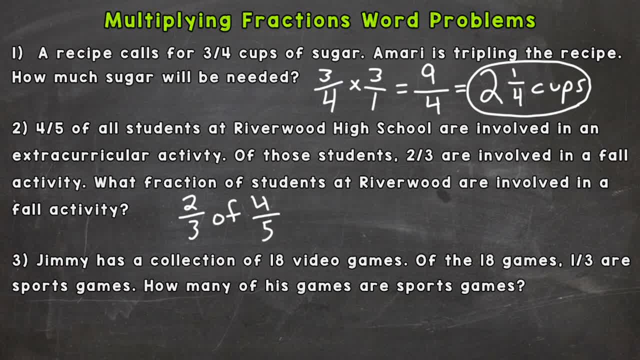 So in this situation, we're taking two-thirds of four-fifths and that will give us our answer, And we can just replace that of with a multiplication sign. We can use multiplication to solve here. So I'm going to rewrite the problem: Two-thirds times four-fifths. 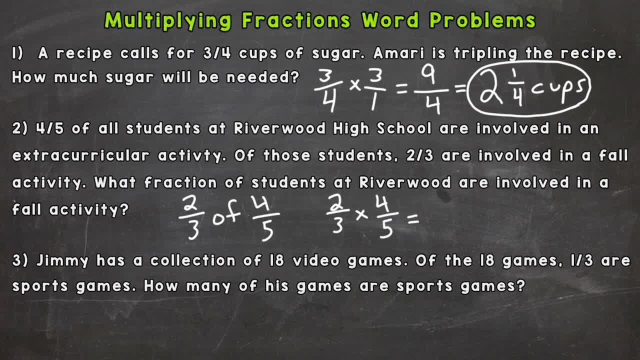 Now I can multiply straight across: Two times four is eight. Three times five is fifteen. That fraction's in simplest form. so now we need to put a label, And our question was what fraction of students at Riverwood are involved in a fall activity? 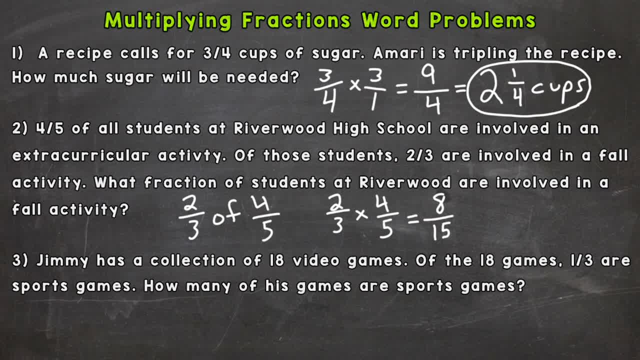 So eight-fifteenths of students are involved in a fall activity. So again, that was a fraction of a fraction type of problem. Now number three is going to be similar to number two, but it's going to involve a whole number and a fraction. 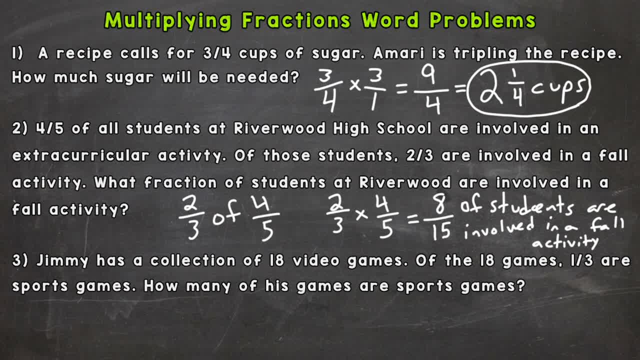 So Jimmy has a collection of eighteen video games. Of the eighteen games, one-third are sports games. How many of his games are sports games? Well, much like number two. we're taking a fraction of something We're taking. one-third of his eighteen video games are sports games.